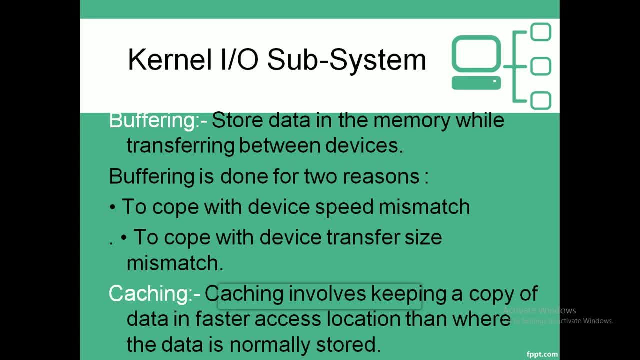 Very essential So that it can cop up with device speed mismatch and cop with the device transfer size mismatch. Caching involves keeping a copy of data. It's keep duplicate data and store duplicate data in memory. Yeah, And buffering and caching is quite similar. 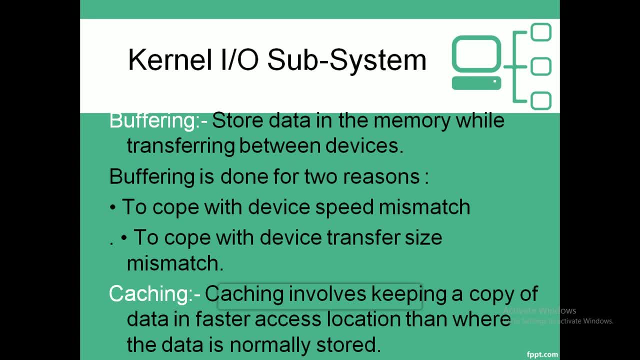 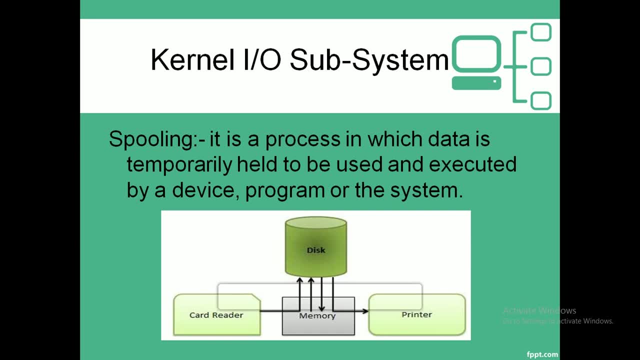 In case of buffering, we store the original data And in case of caching, We store the duplicate copy of data, Spooling. So spooling, it is a process in which data is temporarily held to be used for executed by a device program. 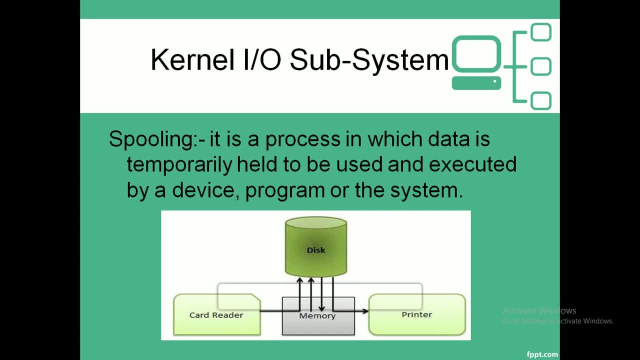 Like if we are inserting, we are using a temporary data, like in this diagram, we are inserting a card reader, So the data from card reader will go to the secondary memory, like disk, and then it will transfer To the main memory And 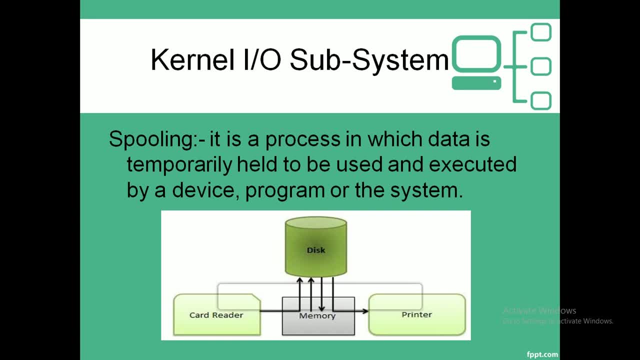 And after execution from main memory It will again store data in disk And whenever it wants to access the hardware devices, like printer, So data will fetch from the secondary memory. Then it will associate to the hardware devices. We use spooling so that a flow can maintain. 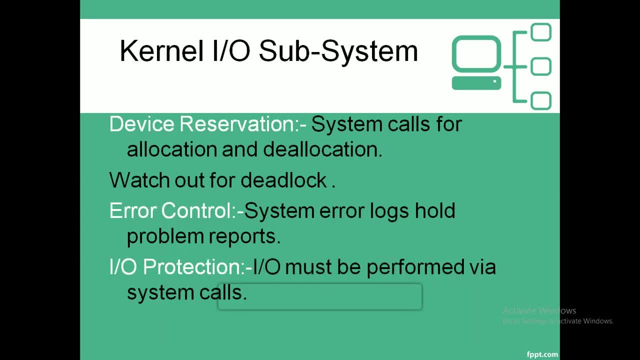 In order to access the hardware devices. okay, so the another thing is device reservation, like I already talked about. the system calls, like if any software or application wants to access hardware devices. so firstly, it will send request to the kernel and it will make system calls and, according to our order of 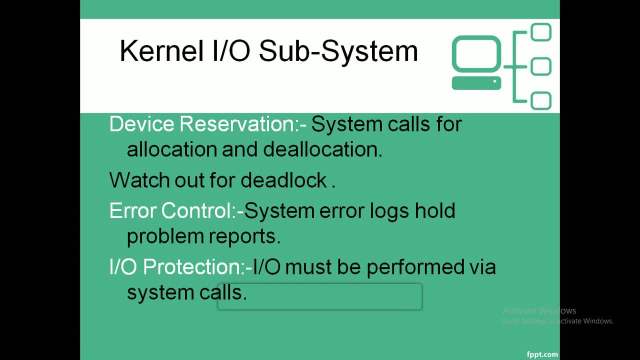 system, call the kernel, will associate hardware devices to the software and application. and another one is error control, so there would be a system error log, so can we, so that we can find the problem reports and we can resolve them. and another one is input output production. so so, in order to reduce any